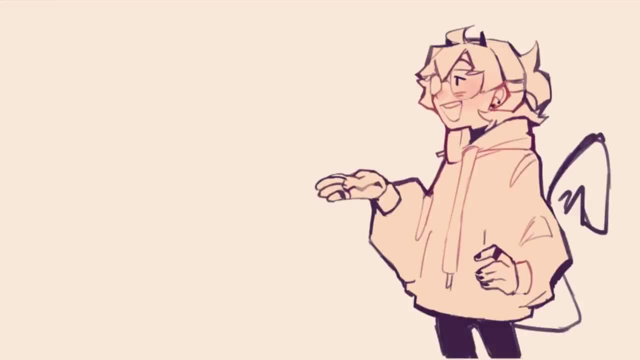 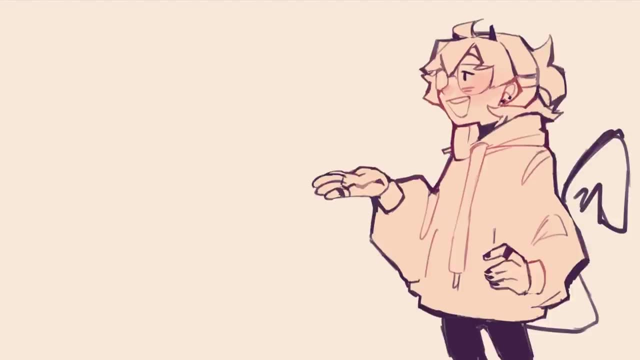 art stuff is called elements of art, which are form, lines, space, colors, texture and value. So I'll be making short video series about the elements of art. These elements of art can be used to help you understand art a lot better and they are very good building. 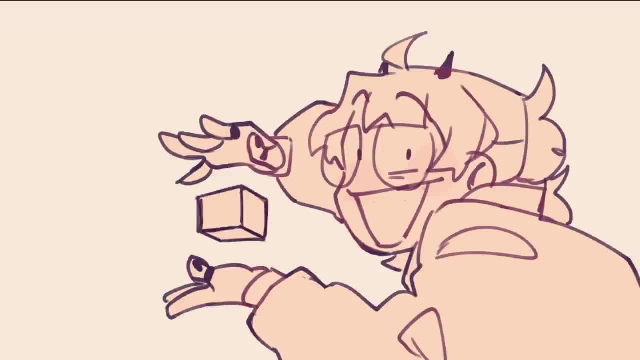 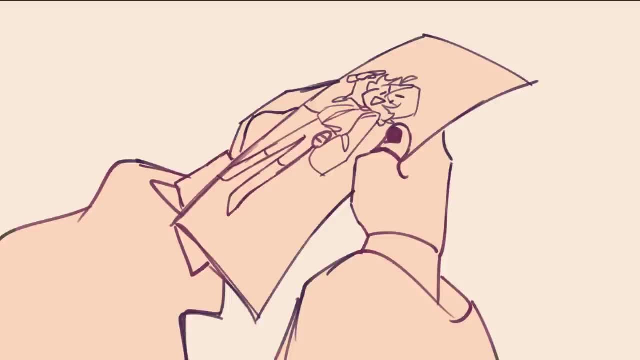 blocks. So today I'll be explaining form. Form is turning a simple shape into a shape that has depth and perspective. When you are drawing on paper or a screen, it's a flat surface, but you're trying to give the illusion of height, depth, width, often through the 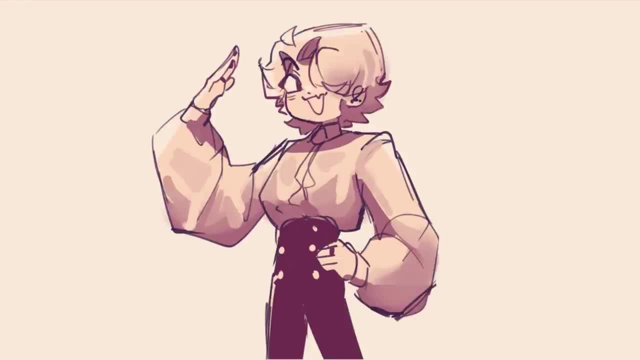 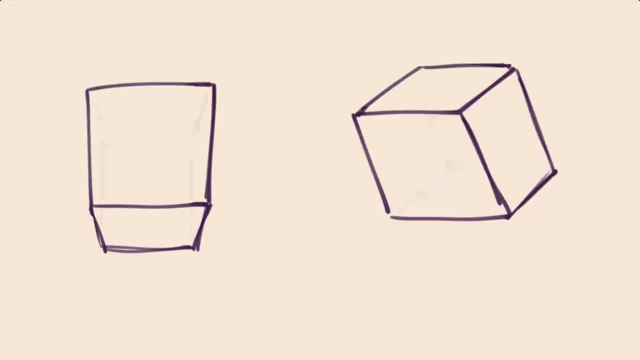 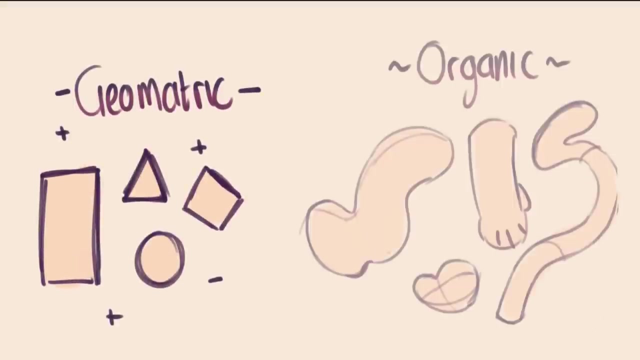 use of lighting, shadows and rendering. For example, this is just a square, but now you can see it's a cube. I added a couple well-placed lines and that gives the illusion of depth. With form, there are two kinds of shapes. There's geometric shapes and then organic. 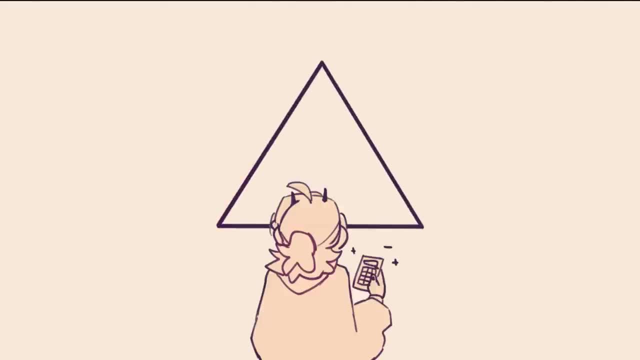 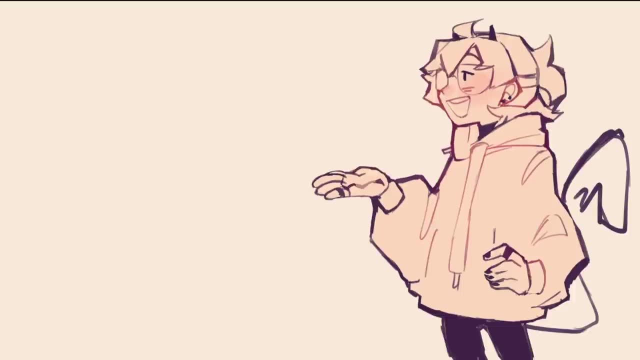 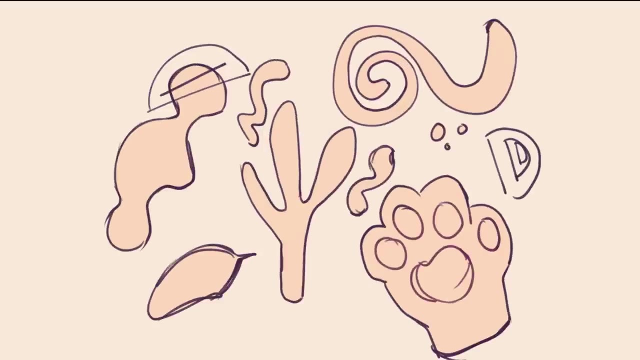 shapes. Geometric shapes are unnatural shapes which are mathematically correct, like cylinders, pyramids, cubes and spheres, So like this. And organic shapes are natural shapes which are normally asymmetric, free-form or curved, So kind of like this. 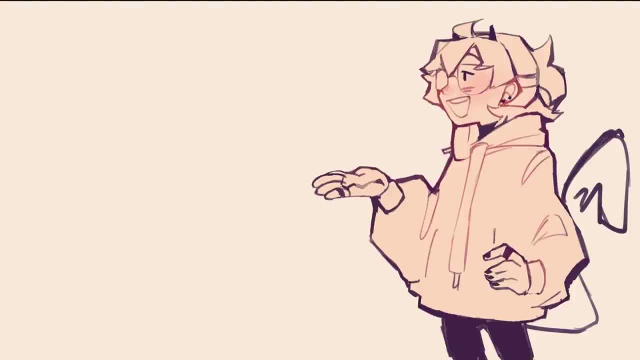 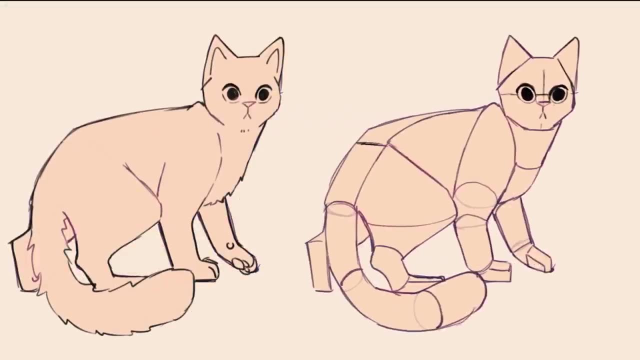 Knowing geometric forms from different angles and perspectives will help you understand and draw organic shapes a lot better. So, for example, this is a cat. This cat can be broken down into basic geometric forms and thus making them a lot easier to draw from different 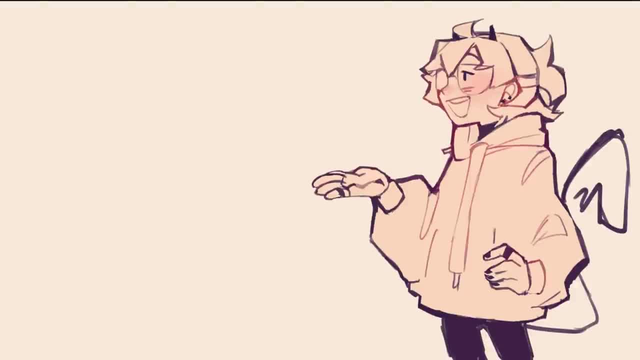 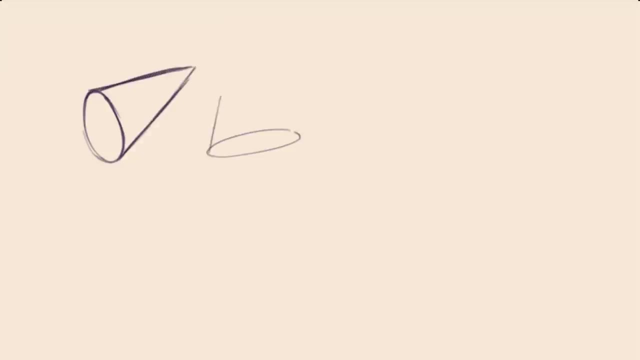 angles and different perspectives. You can start practicing form by drawing different geometric shapes from different angles and perspectives. You can start out with a simple shape and then try drawing them from different angles and perspectives. When you're drawing a geometric shape with depth and perspective and whatever. 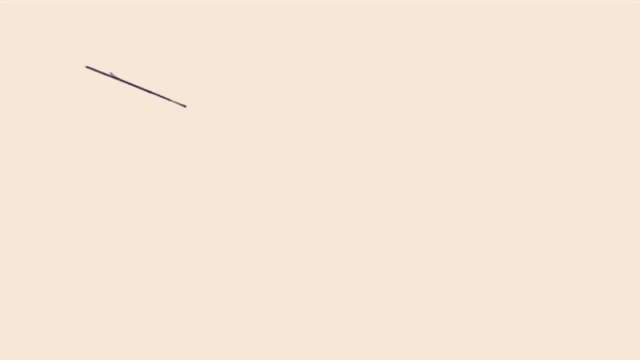 try imagining all corners and all sides and then drawing that into the drawing. I know they seem a little bit silly to be drawing shapes like this, but getting familiar with the 3D shape and drawing them is a lot of fun. I hope you enjoyed this video and 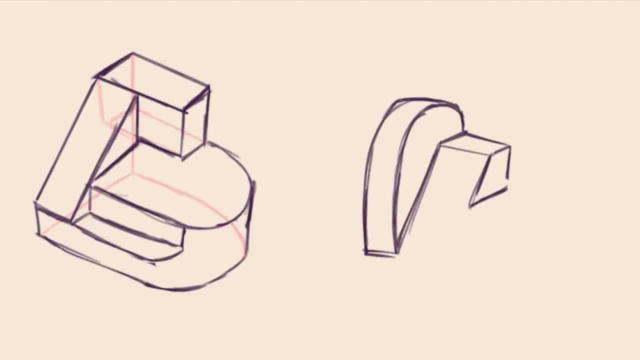 I'll see you in the next one. Bye. And being able to imagine them and draw them from your head will make drawing a lot easier, especially to be able to imagine like a 3D scenario or a 3D picture and be able to put 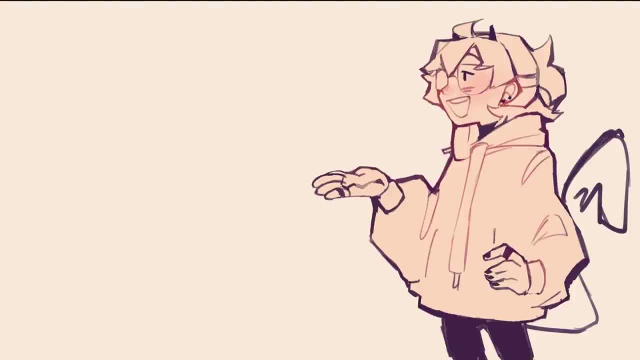 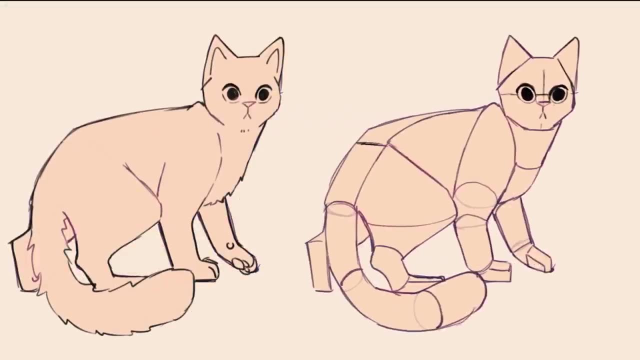 Knowing geometric forms from different angles and perspectives will help you understand and draw organic shapes a lot better. So, for example, this is a cat. This cat can be broken down into basic geometric forms and thus making them a lot easier to draw from different 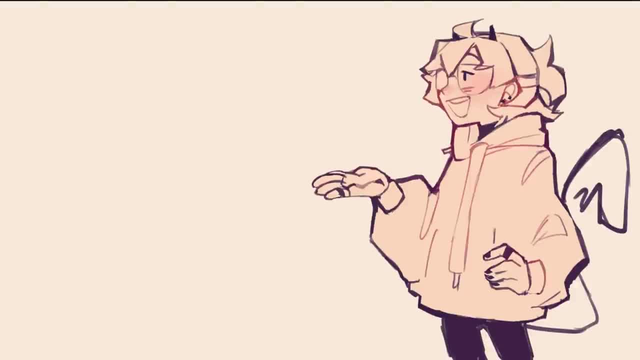 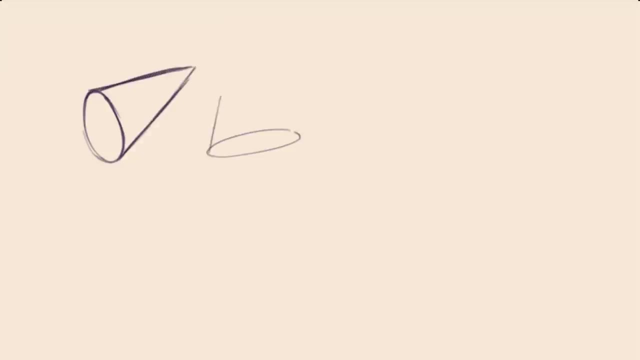 angles and different perspectives. You can start practicing form by drawing different geometric shapes from different angles and perspectives. You can start out with a simple shape and then try drawing them from different angles and perspectives. When you're drawing a geometric shape with depth and perspective and whatever. 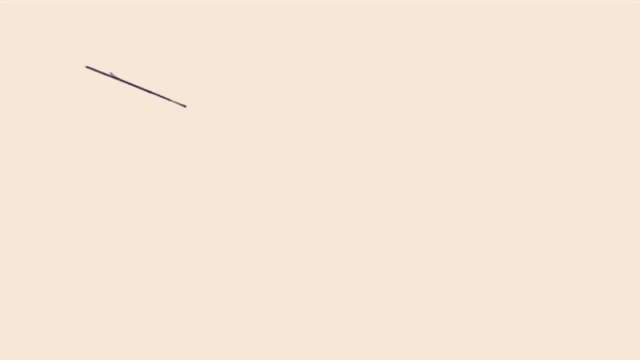 try imagining all corners and all sides and then drawing that into the drawing. I know they seem a little bit silly to be drawing shapes like this, but getting familiar with the 3D shape and drawing them is a lot of fun. I hope you enjoyed this video and 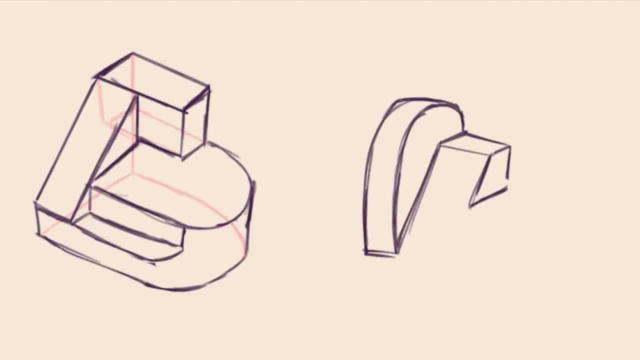 I'll see you in the next one. Bye. And being able to imagine them and draw them from your head will make drawing a lot easier, especially to be able to imagine like a 3D scenario or a 3D picture and be able to put 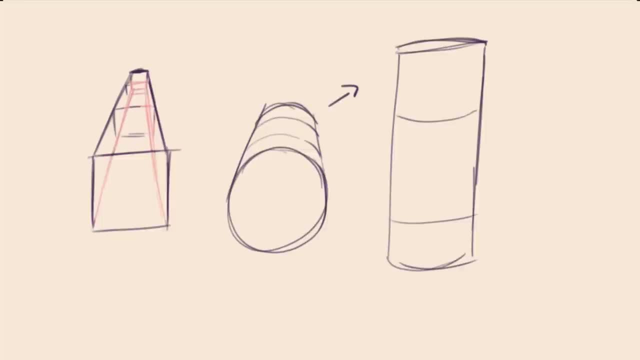 that onto the paper. I promise, Just do like a couple of them every now and then. just keep them familiar. Try and be aware of the depth of your shape. How big is it? How short is it? How far is it? Which angle are you looking at it? 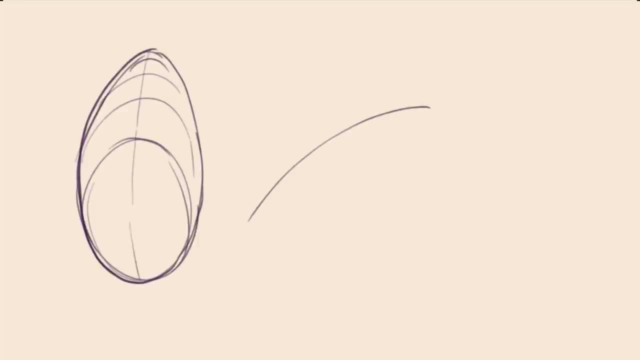 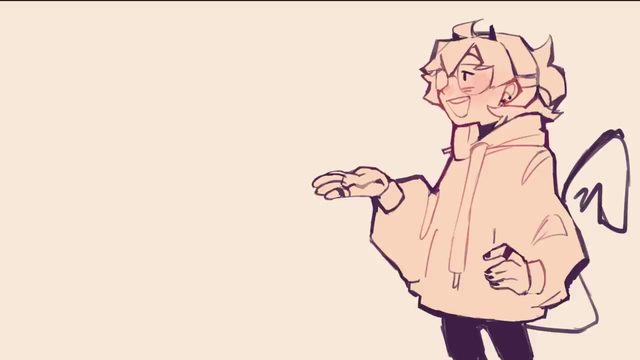 You can feel free to redraw the ones I'm drawing on the screen right now. I'll have a lot more linked down in my description of the ones I drew. Feel free to download them and redraw them if you want. Next you can move on to organic shapes practice. You can start with a random shape, like I have. 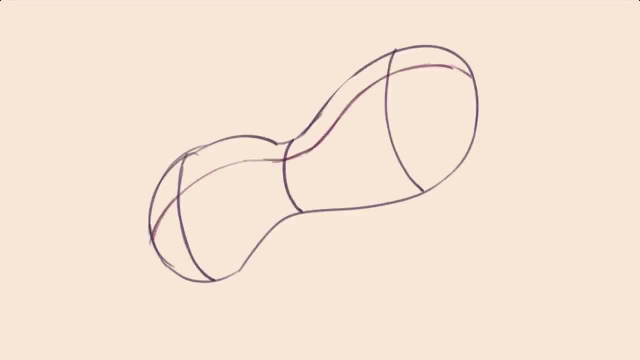 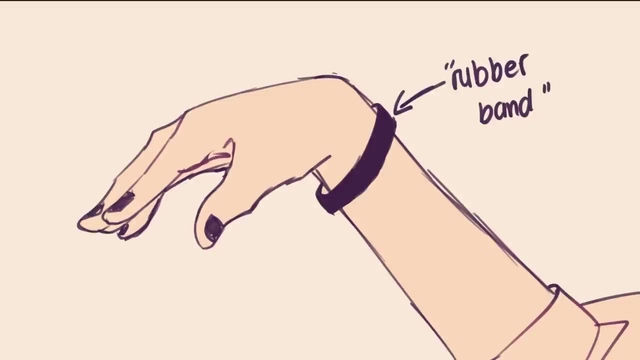 here, Find the center line. so remember that center line is the middle part of your form, And then you can move on to something that's called rubber bands, which is a rubber band essentially, So it's a line that wraps around a shape. This will help. 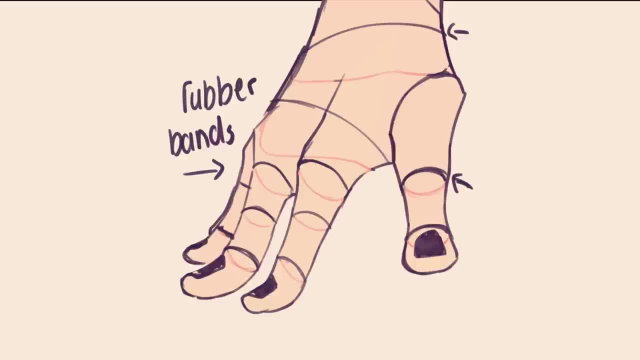 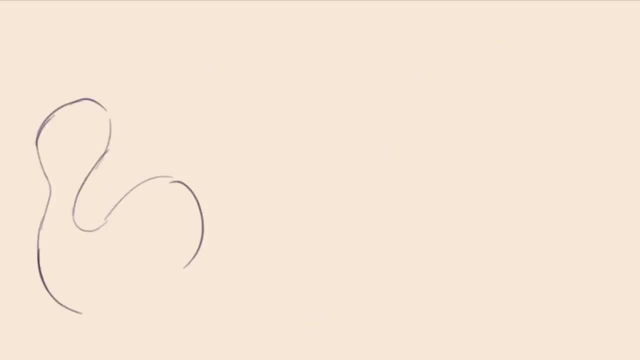 you imagine all angles of this. It will also make it easier to understand the width of your shape, the depth and all that stuff. So here I have more organic shapes that I've drawn. I kept the middle line and I've kept the rubber bands. You can tell that there's like different kind of shapes here. So there's. 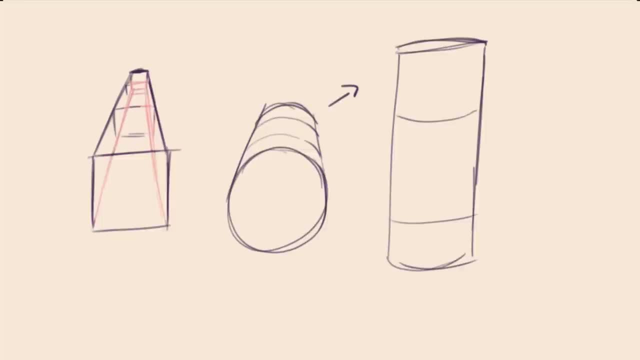 that onto the paper. I promise, Just do like a couple of them every now and then. just keep them familiar. Try and be aware of the depth of your shape. How big is it? How short is it? How far is it? Which angle are you looking at it? 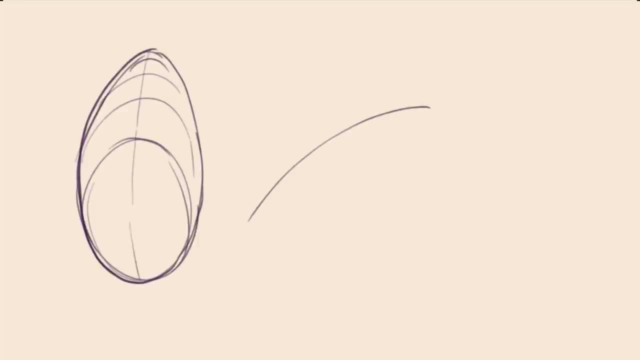 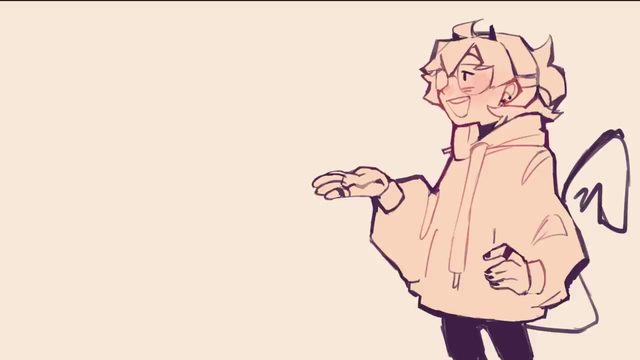 You can feel free to redraw the ones I'm drawing on the screen right now. I'll have a lot more linked down in my description of the ones I drew. Feel free to download them and redraw them if you want. Next you can move on to organic shapes practice. You can start with a random shape, like I have. 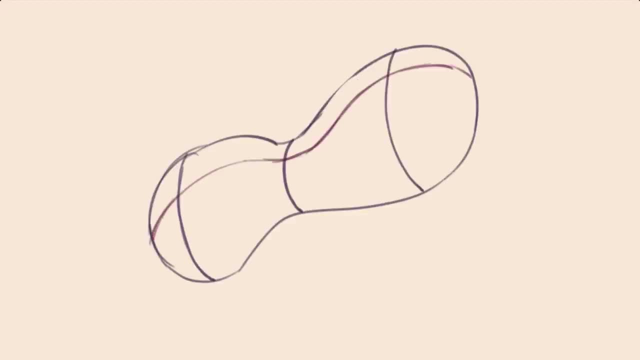 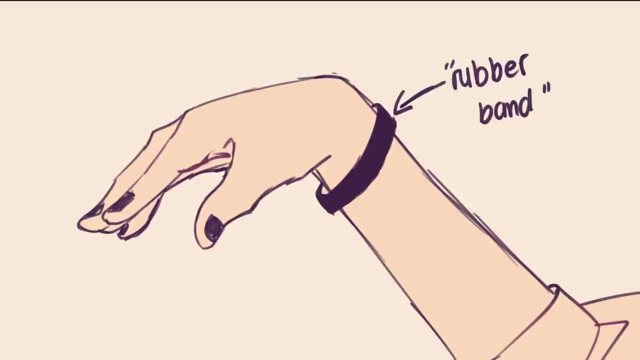 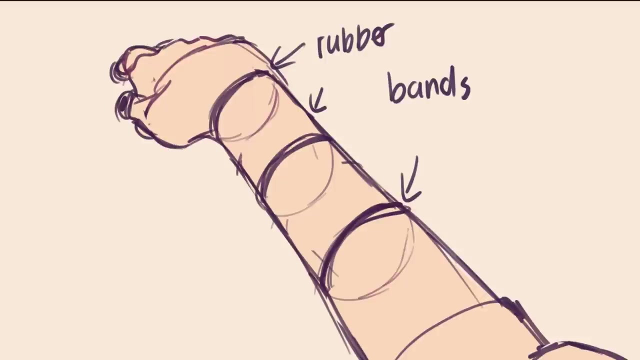 here, Find the center line. so remember that center line is the middle part of your form, And then you can move on to something that's called rubber bands, which is a rubber band essentially, so it's a line that wraps around a shape. This will help you imagine. 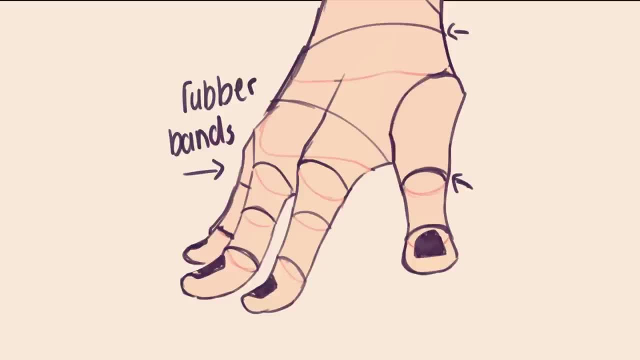 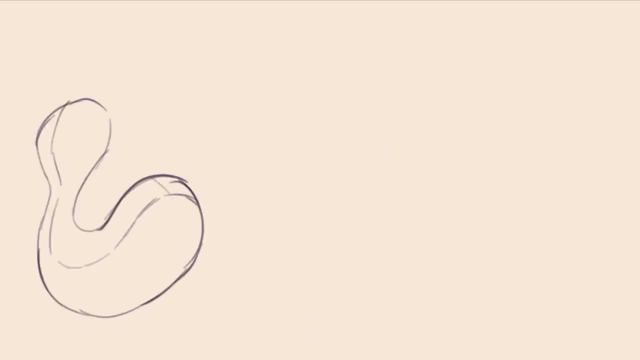 all angles of this. It will also make it easier to understand the width of your shape, the depth and all that stuff. So here I have more organic shapes that I've drawn. I kept the middle line and I've kept the rubber bands. You can tell that there's like different kind of shapes here, So there's. 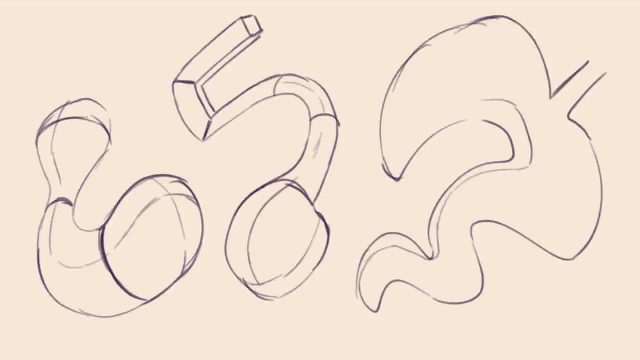 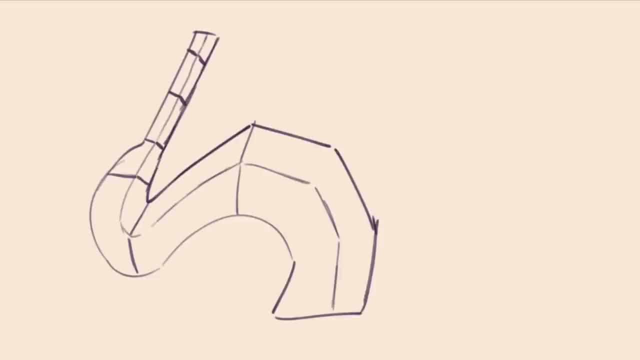 a wider circle or a smaller one or sometimes kind of like an oval shape. I just kept it very natural, asymmetrical, just very flowy. I guess The final practice would be combining organic shapes and geometric shapes by doing these four steps. 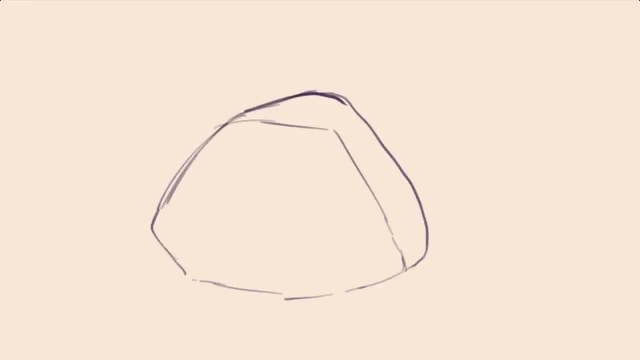 So the first one would be interlocking. This would be practicing shapes kind of sticking to each other, like kind of what I'm doing here. This could be used in practice when you draw hands, like fingers attaching to a palm, because that's the two shapes you're. 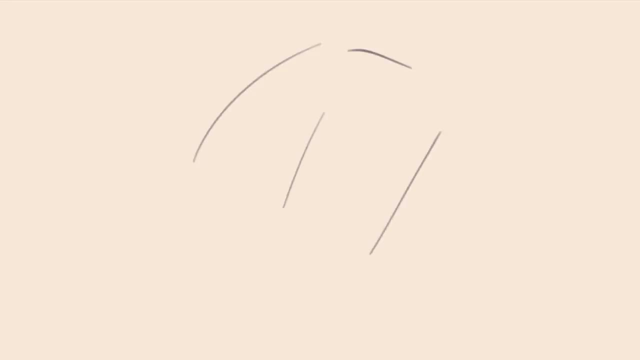 connecting. It's a square connecting to your cylinder, Or if you're connecting an arm to a torso. that's another example. The second practice would be drawing shapes penetrating each other. I don't mean it like that, I mean it as in shapes, kind of like interacting with each other, So like a hand. 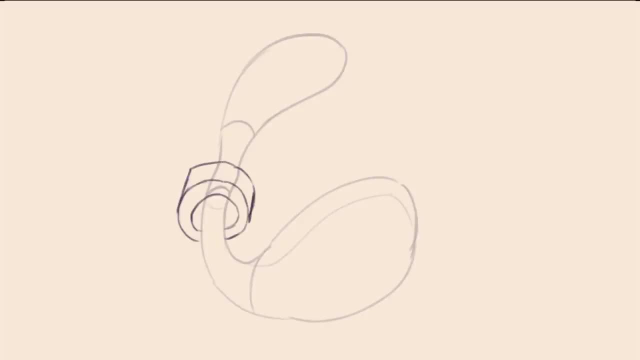 wrapping around an arm, right, That's just cylinders wrapping around another cylinder in basic form. But if you know that and you're able to picture that, it helps a lot with drawing and like getting down a basic sketch. So just practicing this will help, you know.